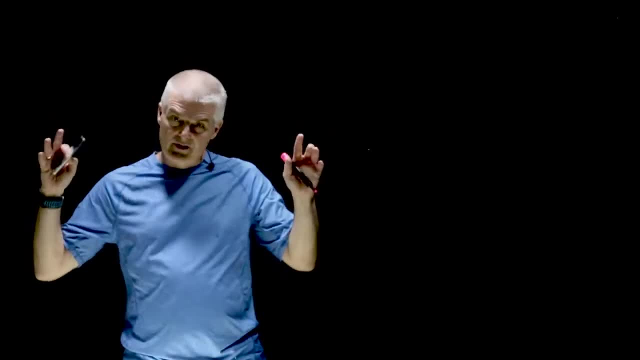 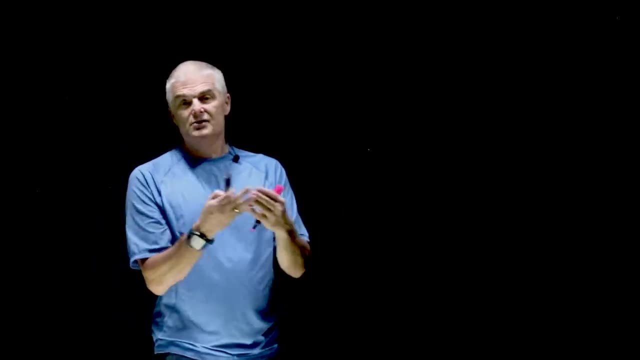 a third time In a mastery-based course. that's the idea is: if you fail, so to speak, you can take it again right. The goal isn't for a grade, but actually it's to learn. So if you fail a test, 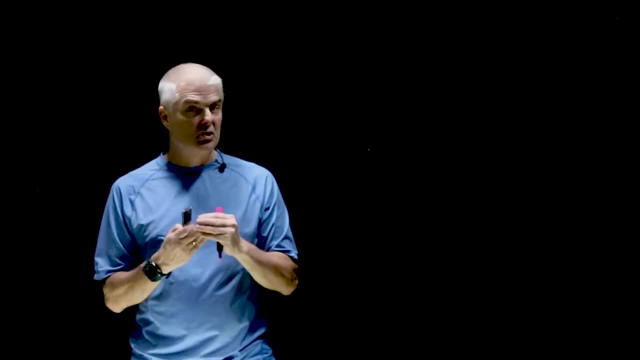 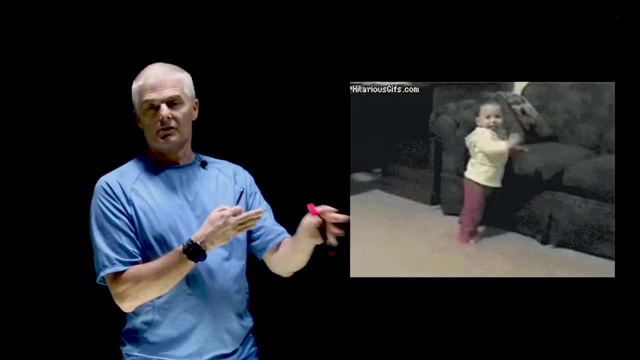 you can take it over, Because I believe that people shouldn't be punished for learning slowly, but rather to see learning as an opportunity to grow. That's, in fact, actually how people learn. You've ever watched a child learning to walk? They first start out by falling. 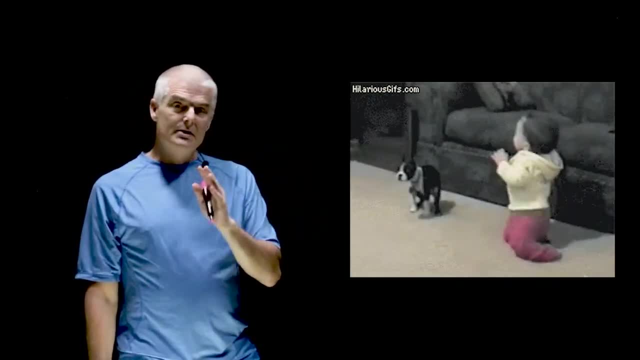 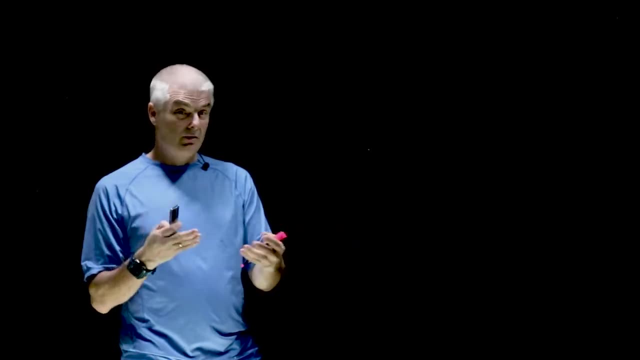 and down, and then they get up and they fall down, and they get up and they fall down. You get the idea. Some people, some kids, they learn slower to walk, but almost everybody learns how to walk. As I'm sure you're aware, science is all about experiment, which is by definition. 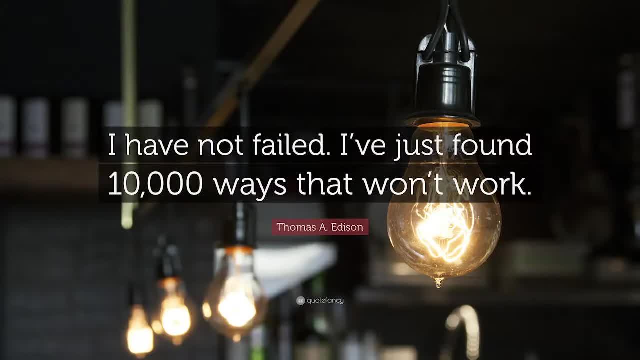 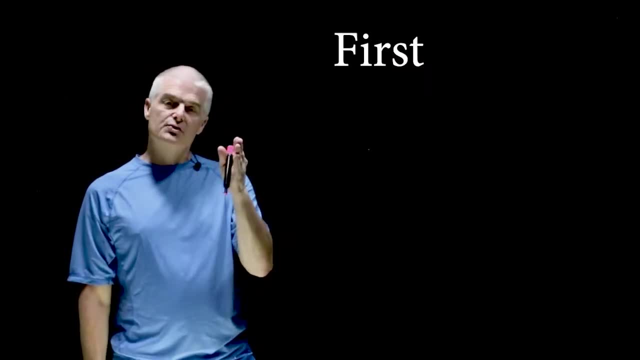 failure. Thomas Edison famously said: I haven't failed. I've found 10,000 ways that won't work. Failure is this. I like to think of this as an acronym. Failure means first attempt in learning. So let's get down to the nuts and bolts. How's this actually? 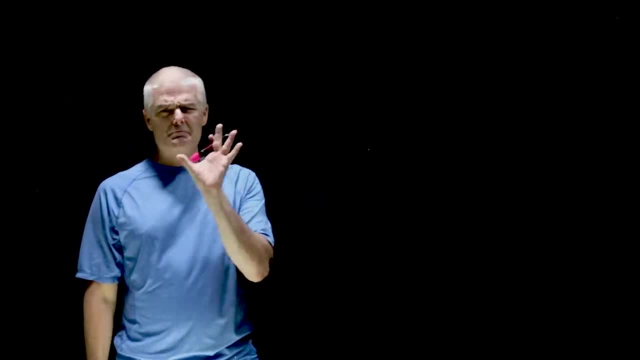 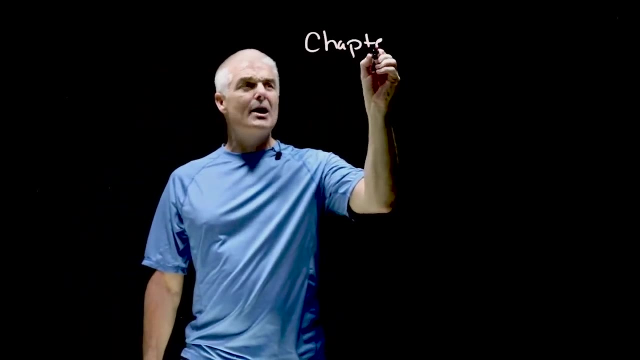 How's this actually going to work in your class? How do I get graded? All that kind of stuff? Big, important questions. So first of all, we're going to use some terminology Now you might have seen the term. I've got to finish the chapter. We don't have chapters, We have. 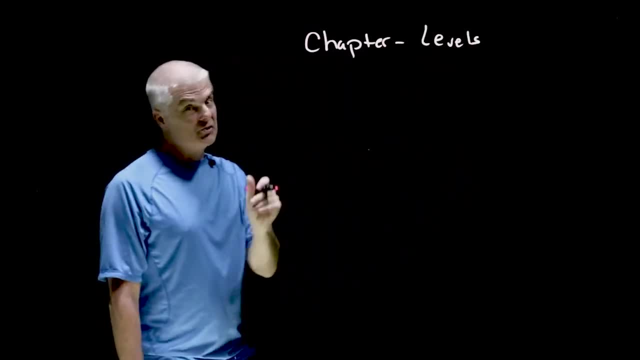 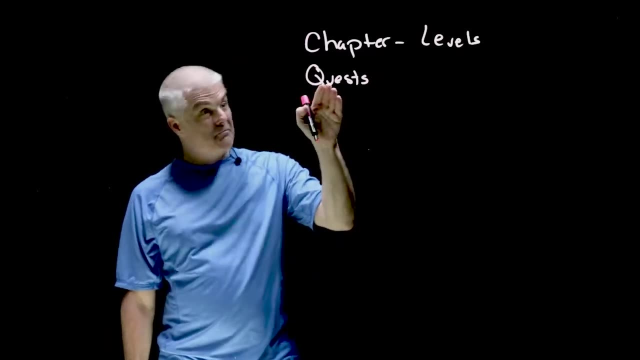 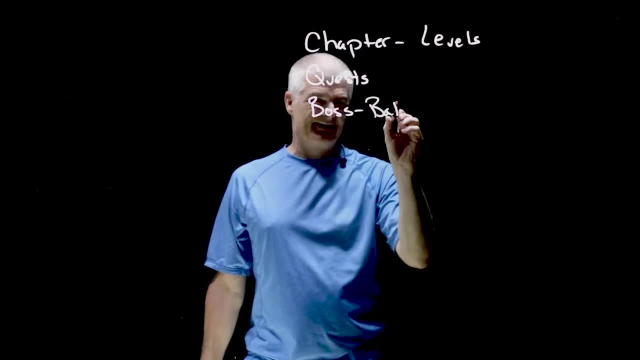 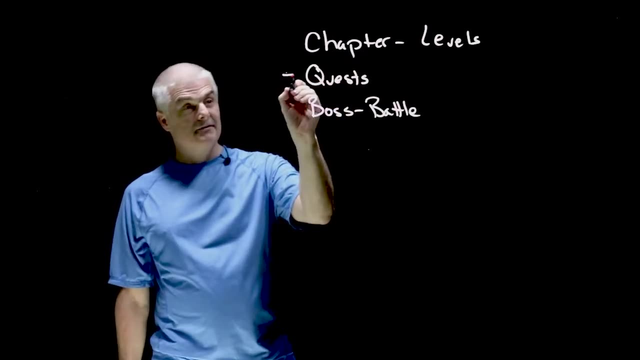 level. We don't call them tests, They're called boss battles because you have to. when you beat the boss in a game, then you level up. That's the idea, And so you're going to do individual quests that lead are part of the full level. Then you get to the boss battle. Now, at the 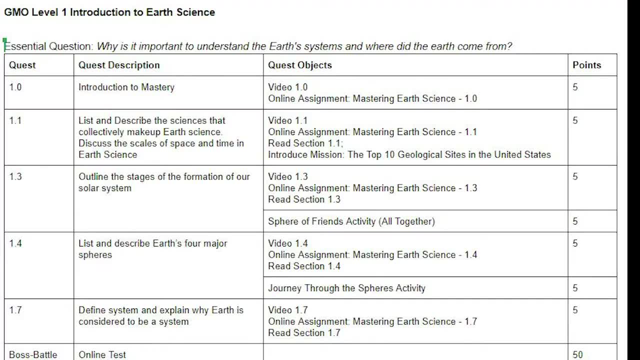 beginning of every unit you're going to get a chart that looks like this. So this is the level one quest map And you might notice we've got quest objects and quest description And right now you are in the middle of quest 1.0, the introduction to mastery And for you to master it. 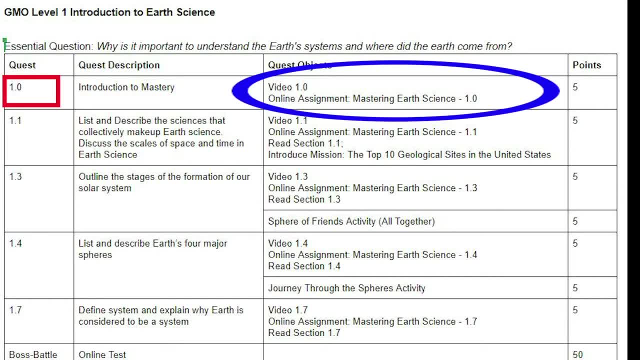 you've got to watch this video, which you're doing right now, take some notes on it, and then you're going to do an online thing in the system, And then you've got quest 1.1.. And, as you can see, 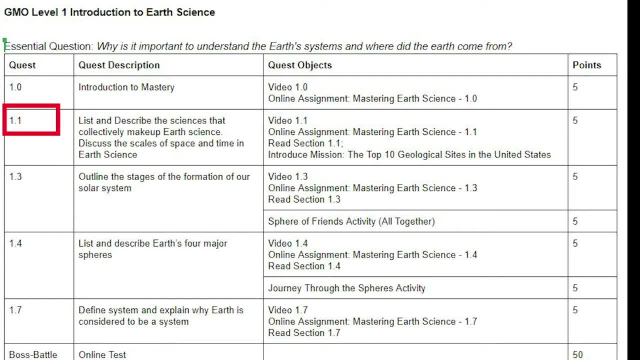 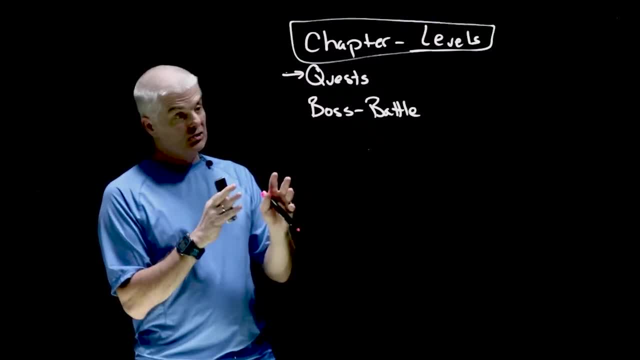 there's a description, et cetera, et cetera, And they're all worth five points. And essentially here's the deal, guys, When you get the end of a particular objective, what you're going to do is you're going to come to me and say, Mr Bergman, I have mastered quest 1.2, or whatever. 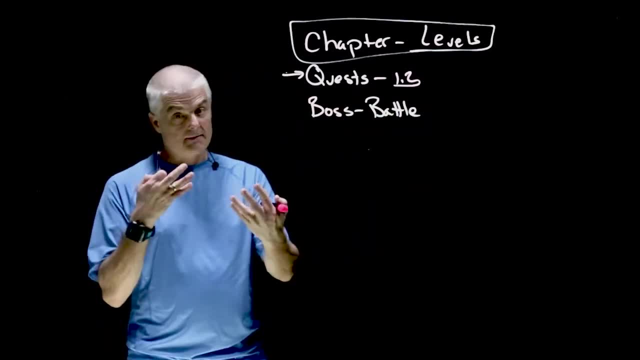 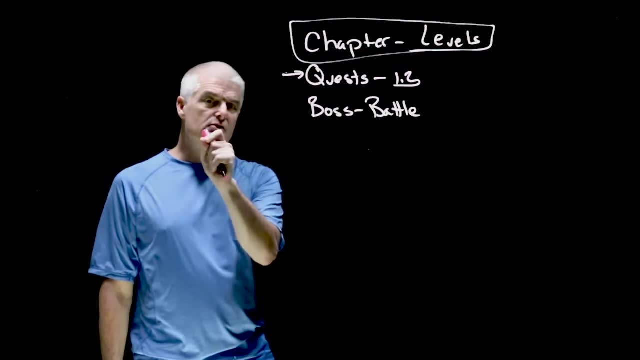 And what you're going to do is I'm going to say: all right, show me your stuff, I'm going to look at it. We're going to have a little conversation, just you and me Conversation. I'll say: you got it Or not quite, You need to do this or that. You'll get the idea. 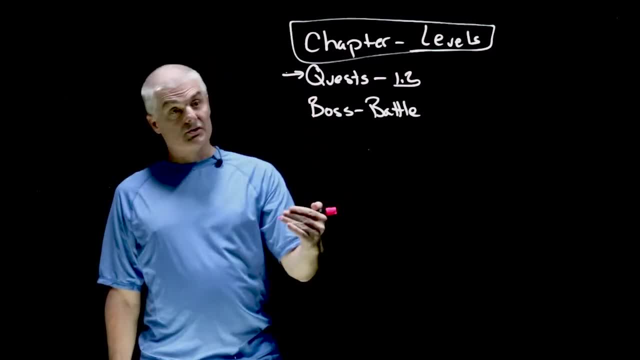 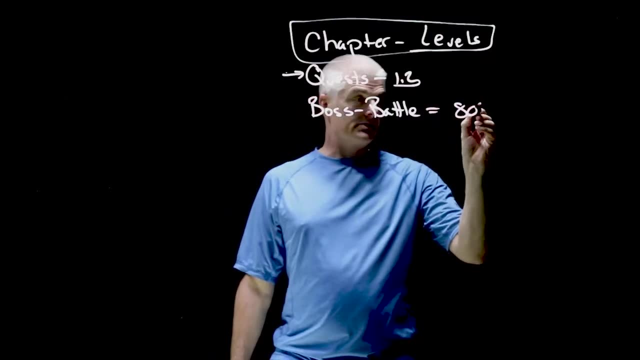 Once you've mastered the quest, you get five points, And then, while all the quests are done, you get to the boss battle. The boss battle is like the test, And on the boss battle- here's the deal: You've got to get 80% or better. Of course, you can get more than 80%. 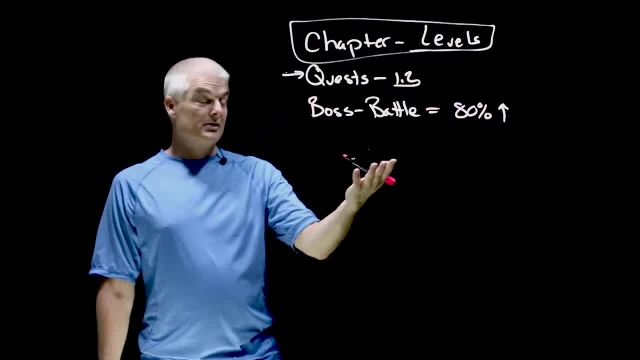 But if you don't get 80%, then you haven't defeated the boss. So that's the deal. You've got to get that. But here's the deal. Don't panic. What happens if you get 65? Like in all? 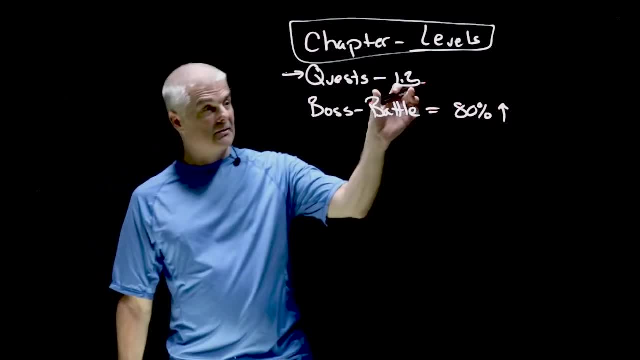 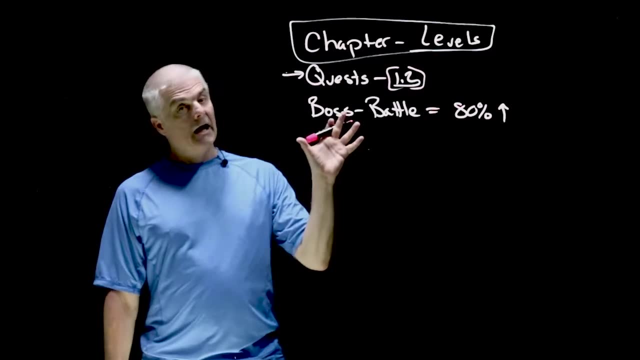 games you can take on the boss again. You have to go back, maybe, and look at some of the quests and say what parts of the quest did I understand, so that when I get back to the boss I can beat the boss. That's the idea of mastery. Let me say this: Some of our levelers are going to have a 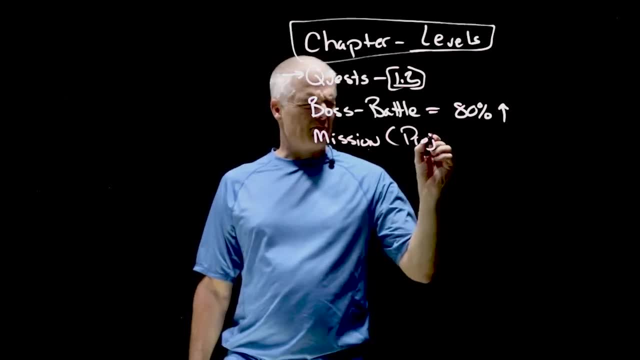 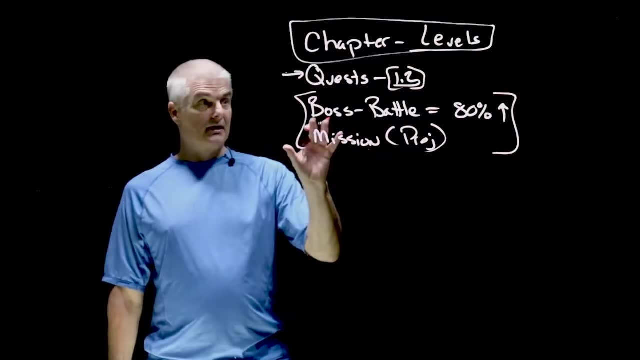 mission. You might think of that old school term. They're called projects And if there's a mission that's part of the boss battle, You have to do both of these. These are the big deals. Now, from a great perspective, I'm going to say: I'm going to do both of these. I'm going to do both of 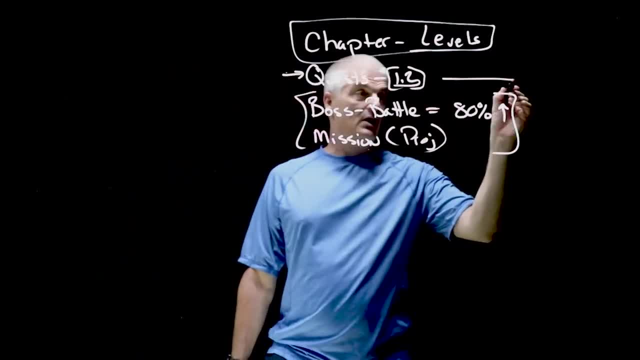 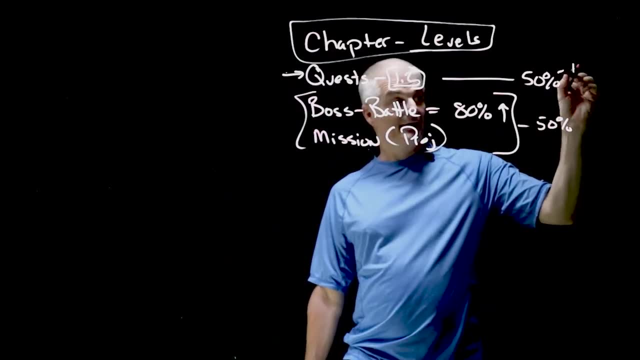 them From a rating perspective. as a side note, the quests are worth 50% of your grade And these are worth 50% of your grade, And if you get 100 on this and you get 85 on this, well, let's say no. 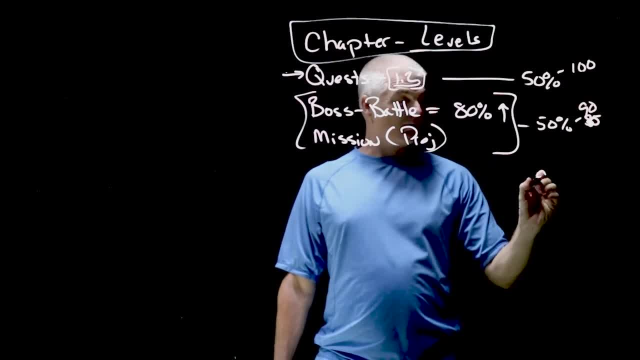 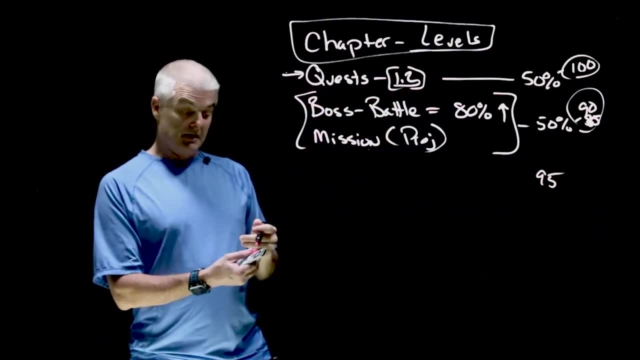 Let's say 90, because it's easier for math. Mr Bergman needs help. Then your score is a 95, 50%, 50%. So whatever your average is for your quests and the averages for these, that's going to be your grade Turns out. the way we do this, very simply, is: at the end of week one, All right. 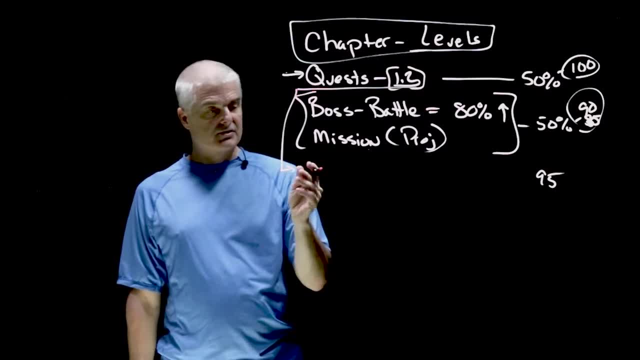 So the average is for your quests and the average is for these. That's going to be your grade. So with the quest, let me say this: you have to do the quests in order. So let's say you do 1.1,. 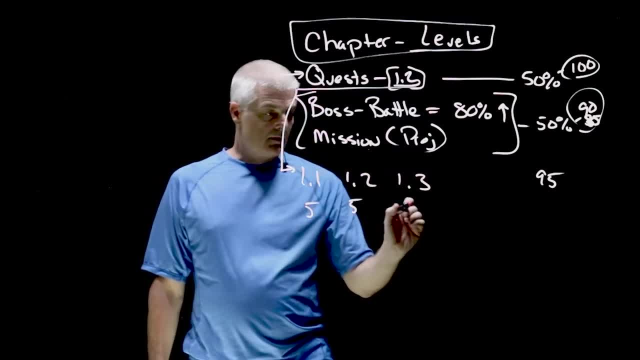 1.2,, 1.3, and they're worth five points. What I'm going to do is I'm going to say, by week one, you've got to get through 1.3. Actually, I think 1.3 might even be worth a total of 10, because 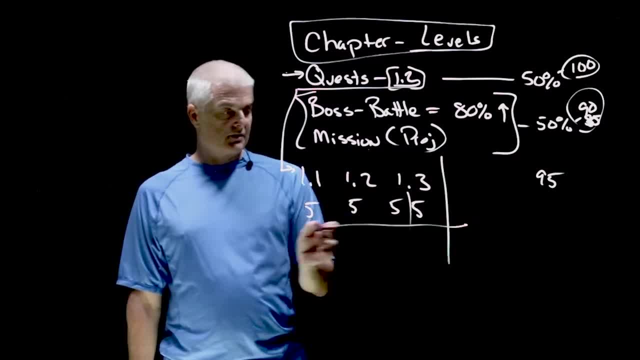 there might be also a lab activity. that's part of the quest, right? So it's out of 20 points. So if you have 20 out of 20, right, that's you 20 out of 20, that's 100, right? So for week one. 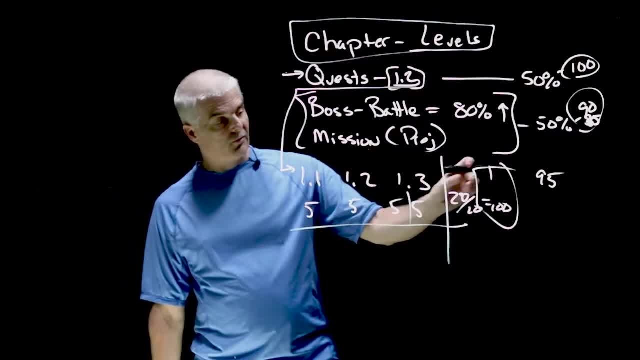 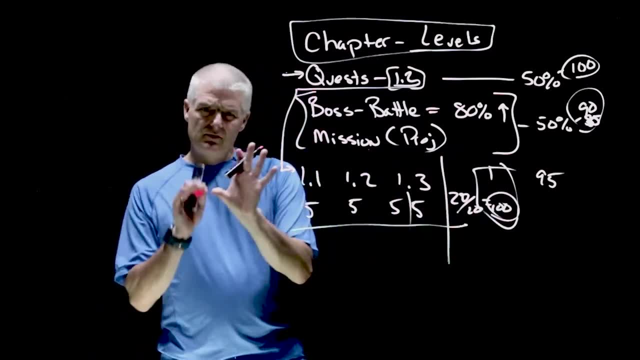 your grade is 100. For week two. now it might include 1.4, 1.5.. Now it's going to be 40 points, And if you get 40, 40, you get 100.. If you get 35 out of 40, you get less, but then you get the average of your scores. If you really 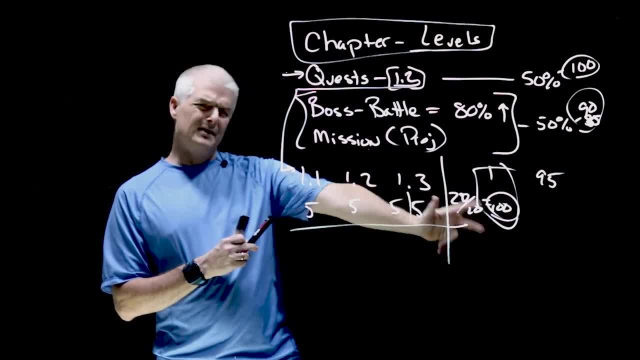 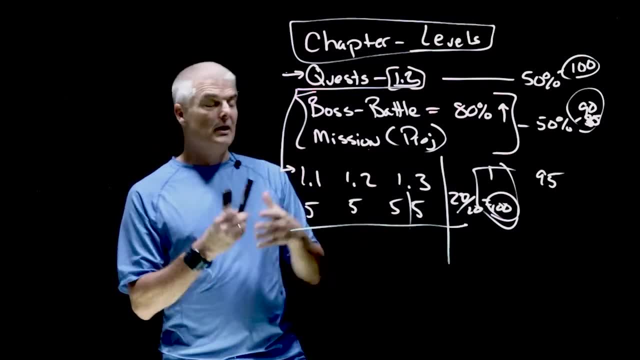 think about this. it's like a built-in late. there's no late work, but there is if you don't complete the required number of quests in a given week, which I'll tell you at the beginning of the week, so you know how to plan your time. Then, when you get to the boss battles, you can take the. 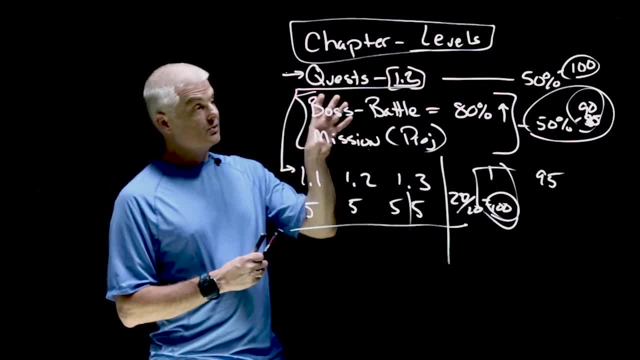 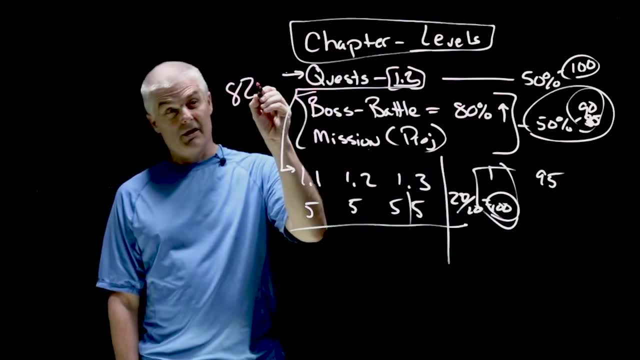 tests, if you will the boss battles as many times as you need until you get the score they want. By the way, some people always ask this: what if I get an 82 on the first test, the first boss battle? Can I retake it Absolutely, If you? 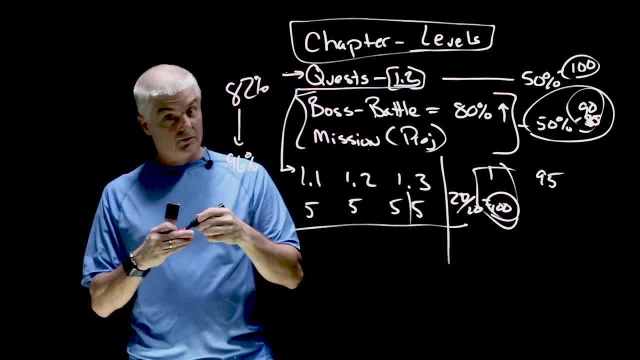 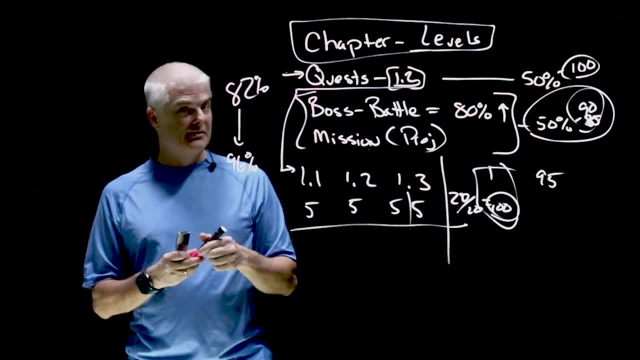 want to score and jump to a 96, go for it Now. as a side note, the test will be different every time you take it. We'll do it completely online in our online system, And so you're going to get completely different tests. So you can't like game the system and try and figure out what that is. 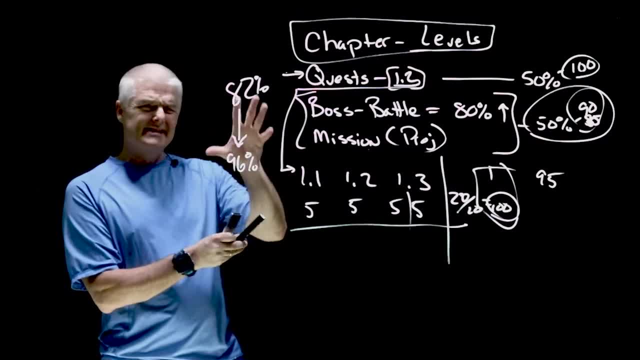 So that's the way the course is going to work. Some of the details we're going to work and what the technology is and where we link to, we're going to get that all set up in class. that you know. So I can't tell you. 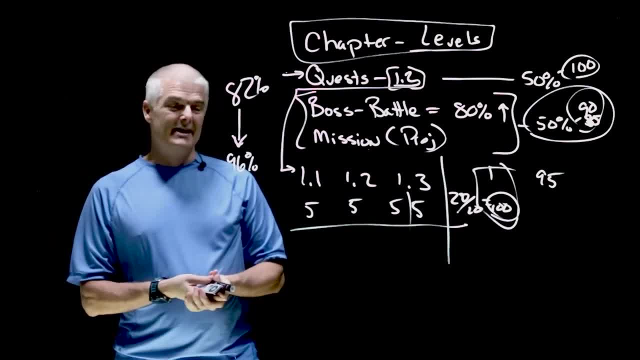 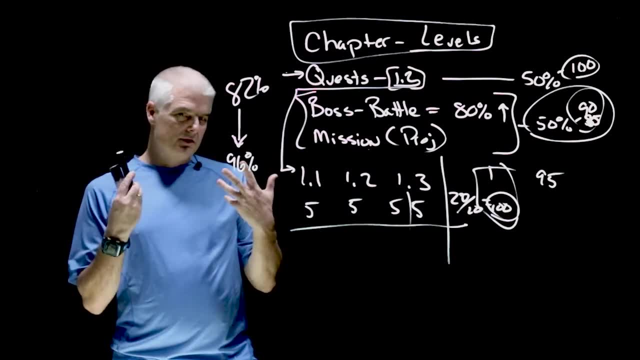 I'm excited I am to be here as your teacher. I'll share more. You can read it in the syllabus that it's been a while since I've been in the classroom, but I've been working with teachers all over the world. It's been awesome to do that. But now I get to be your teacher and I'm thrilled I am. 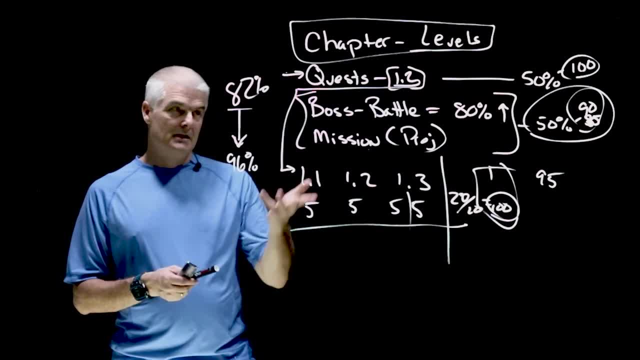 totally, absolutely thrilled to be with you guys this year. Welcome, Welcome to science. We will see you in Classical Houston. We don't got no problem.